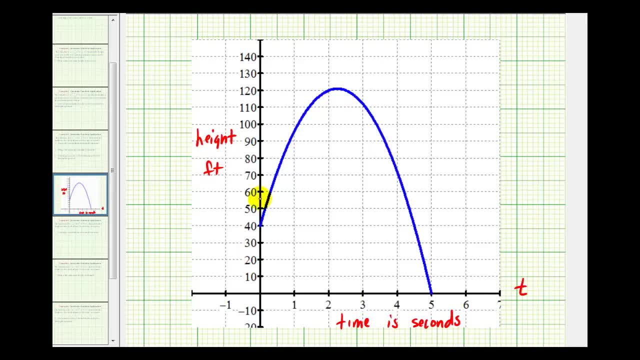 So we can almost answer all these questions from the graph, but we can see that the ball is thrown at this instant, when the time is equal to zero. We can see the initial height would be 40, then it goes up, which is the maximum height here, which would be the 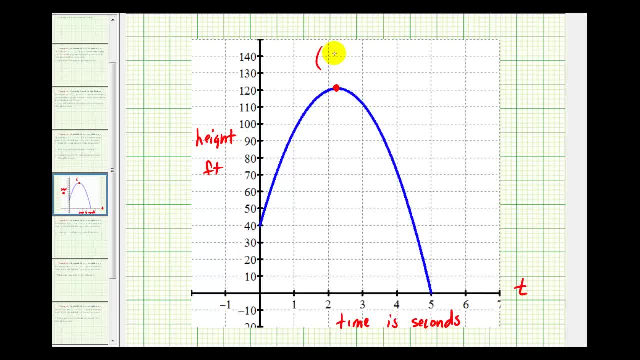 vertex of the parabola. Remember, the coordinates of the vertex are negative b over 2a comma. in this case it would be h of negative b over 2a. And then here is where it hits the ground and we can see it's going to hit the ground. 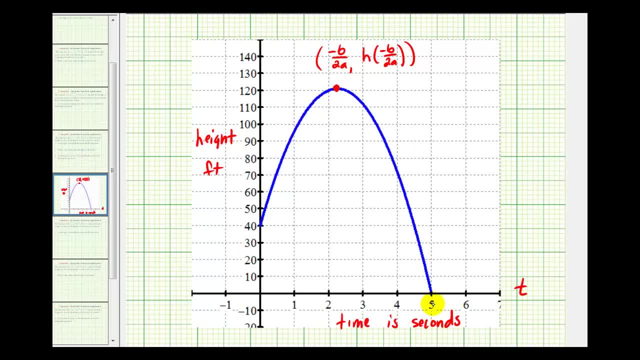 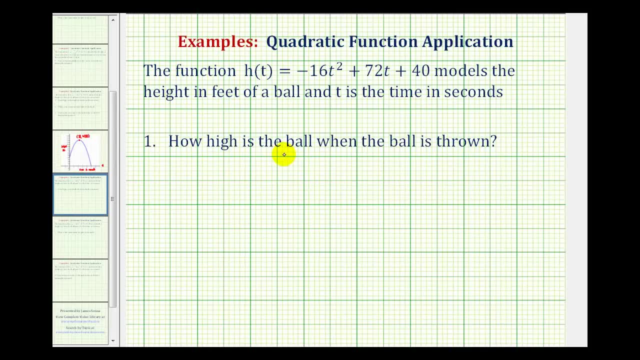 at five seconds. But let's take a look at the simulations to determine these values. First, to determine how high the ball is when the ball is thrown. at the instant the ball is thrown is when the time starts. So if we set t equal to zero, we can find the initial height. 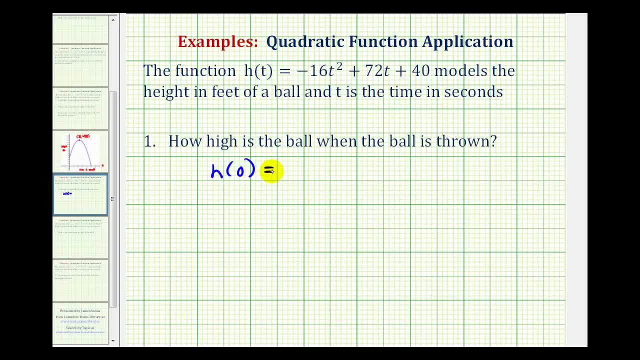 So if t is equal to zero, h of zero would be the initial height, which would be negative sixteen times zero squared plus seventy-two times zero plus forty, which we can see would just be zero plus forty or forty feet, Which again we saw from the graph. the initial height was forty feet. 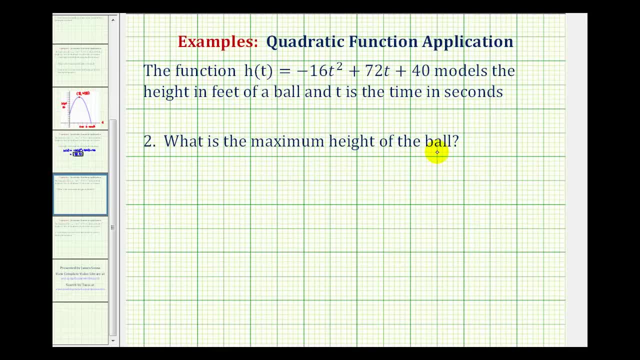 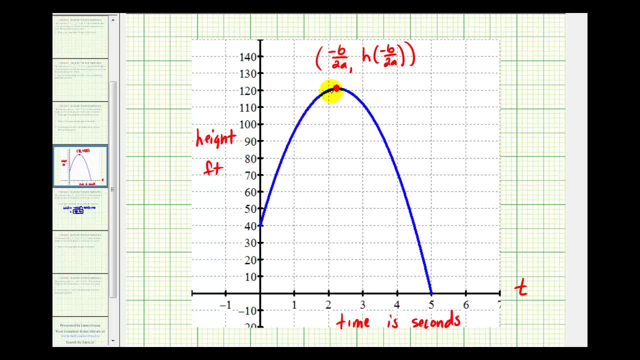 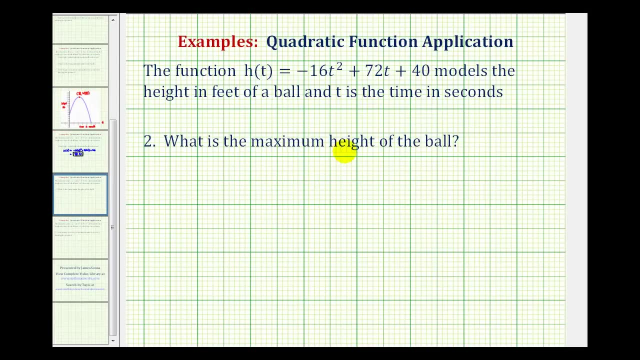 The second question is to determine the maximum height of the ball, which, remember, would occur at the vertex, where the x-coordinate or the t-coordinate would be the time it takes to reach the maximum height And the y-coordinate would actually be the height of the ball. 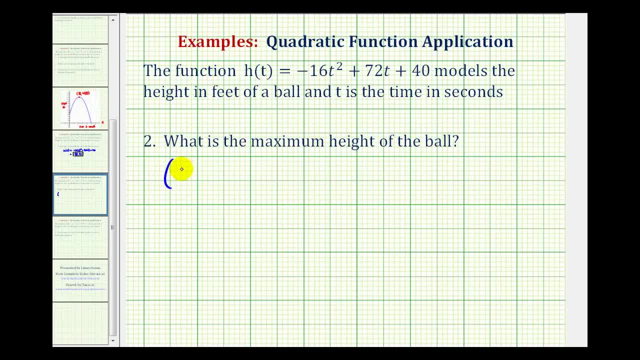 So to determine the y-coordinate of the vertex, we first have to determine the x-coordinate, or in this case the t-coordinate, And then we'll evaluate the function at that value of t. So, looking at our function, a is equal to negative sixteen. 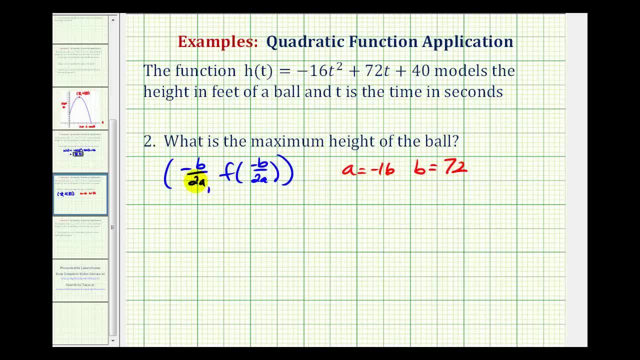 and b is equal to seventy-two. So the x-coordinate or t-coordinate would be equal to negative seventy-two divided by two times negative sixteen, which would be negative seventy-two, divided by negative thirty-two, which comes out to exactly two point two five. 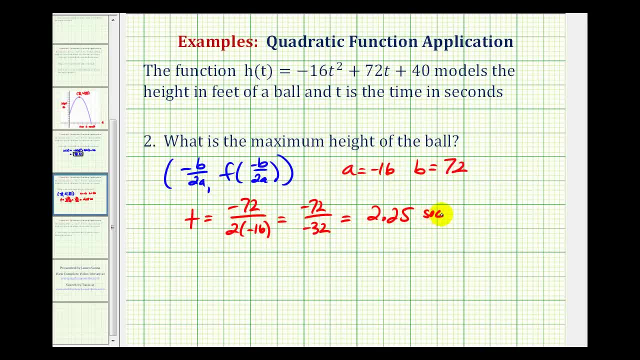 which, again remember, is times. this is seconds. This is how long it takes for the ball to reach the maximum height. but the question asks for the maximum height. Now we need to find h of two point two five, So we'll have negative sixteen times two point. 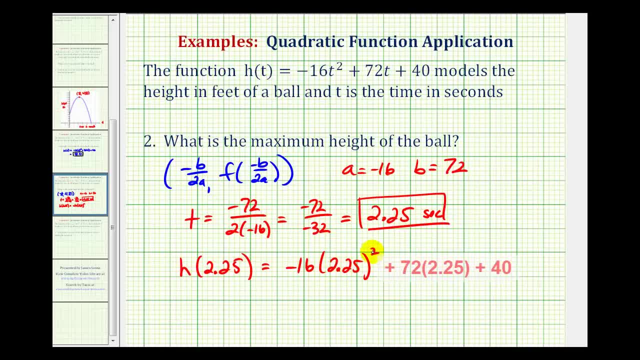 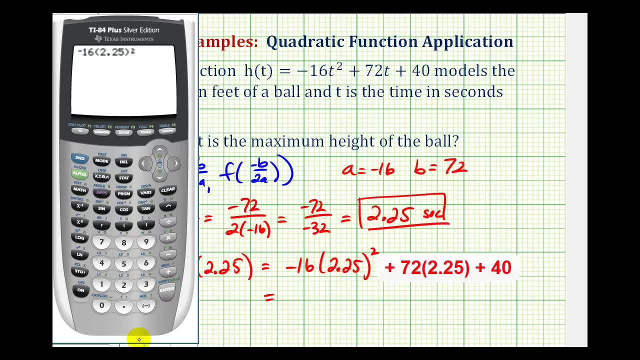 two, five squared plus seventy-two times two point two, five plus forty. And now we'll use the calculator, So we'll have negative sixteen times two point two, five squared plus seventy-two times two point two, five plus forty. So the maximum height is one hundred twenty-one feet. 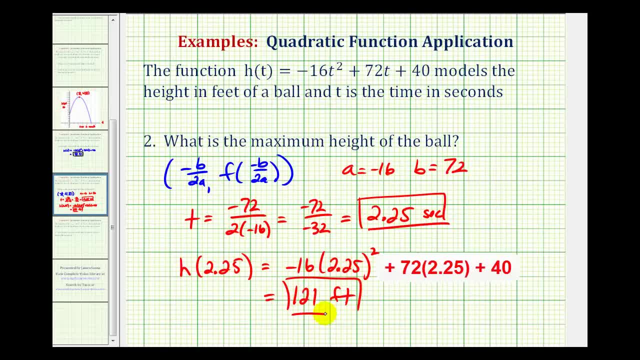 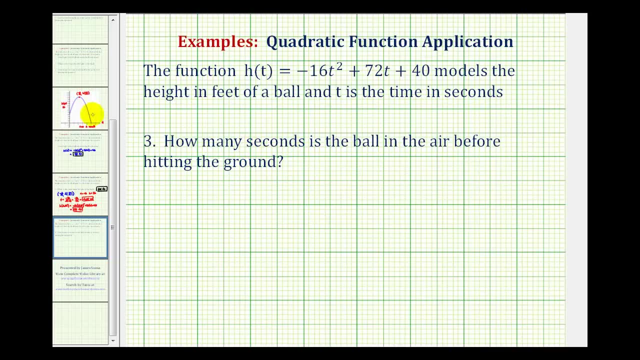 Which is the answer we're looking for. Okay, and then for the third question, we want to know how many seconds the ball is in the air before hitting the ground Again. going back to the graph, we can see it's equal to five. but let's take a look at the 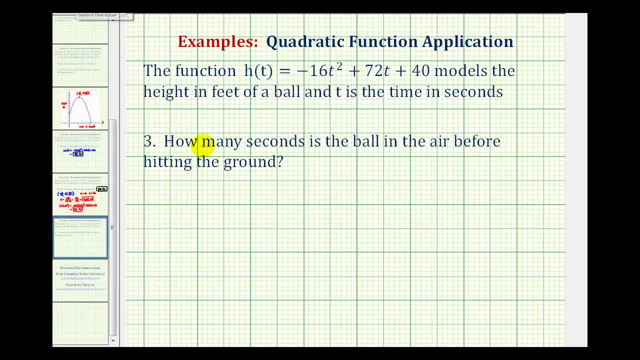 algebra behind this. When the ball hits the ground, the height would be zero, or h of t would be equal to zero. So to answer this question algebraically we'd have to solve the equation: zero equals negative, sixteen t squared plus seventy-two t plus forty. 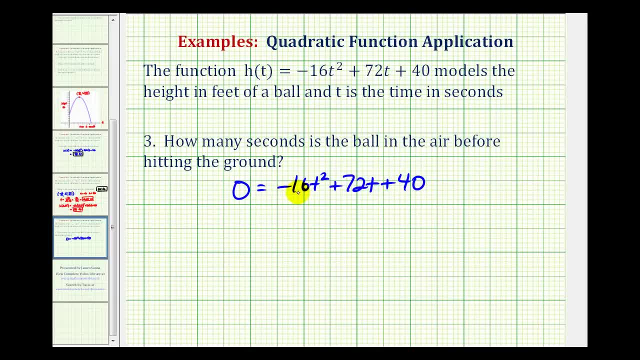 Let's see if we can factor this. We'll first factor out the greatest common factor of eight, But if we want the coefficient to be positive, let's factor out negative eight. That will leave us with positive two t squared minus nine t and then minus five. 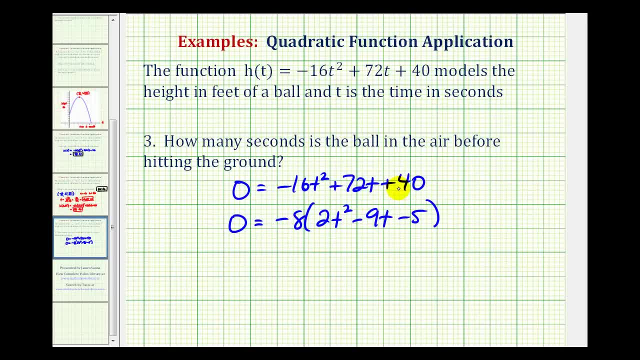 Remember, if we factor out a negative it's going to change the sign of each term. So if this does factor, we'll factor into two binomial factors. The first terms must come from the factors of two t squared, that would be two t and. 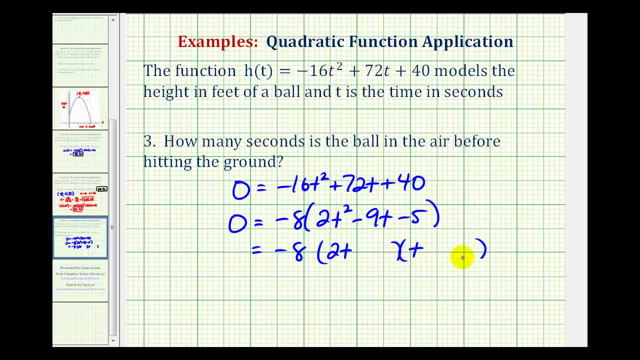 t. The second terms must come from the factors of negative five, so that the sum of the inner product and outer product would be negative nine t. Notice, if we put minus five here, we'd have to put a positive one here. The outer product.